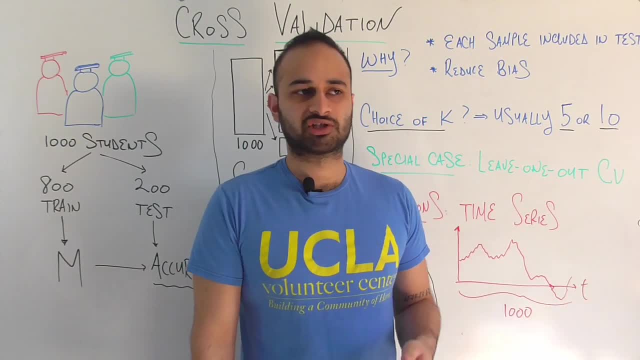 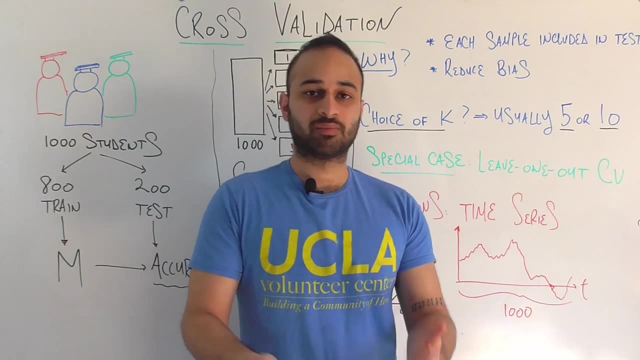 their grades would be better. Sometimes it's not about grades at all. Sometimes they just don't find an interest in this current major and want to make a transition. But either way, we wanted to identify these students one quarter or semester early so that we could better help guide their transition. 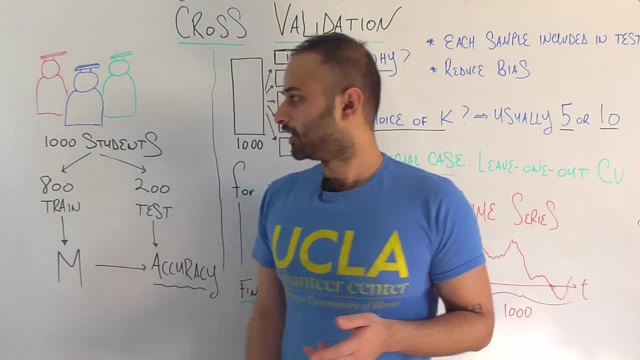 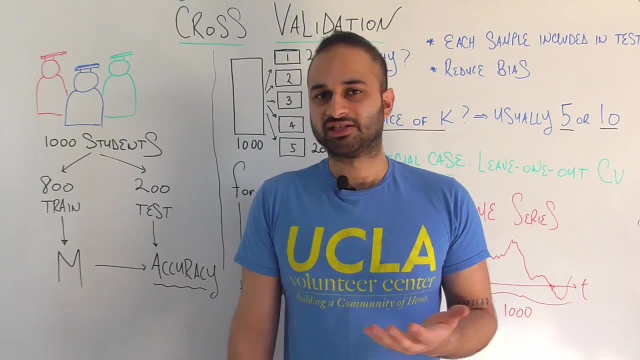 So in the spirit of that example, let's say that there was a thousand students and we're just gonna go down the typical machine learning pipeline- nothing too fancy here, and we'll see why there might be something lacking with this basic idea. So we have a thousand students. Let's say that we do a 80-20 split. So we 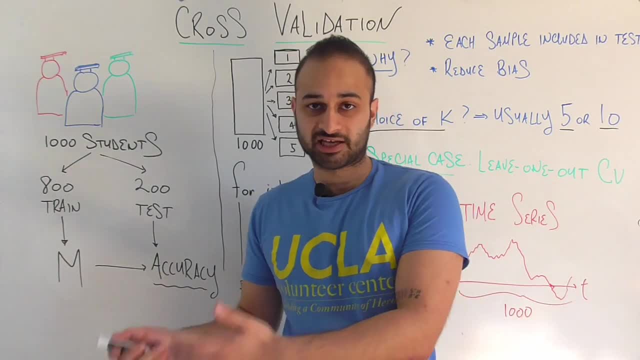 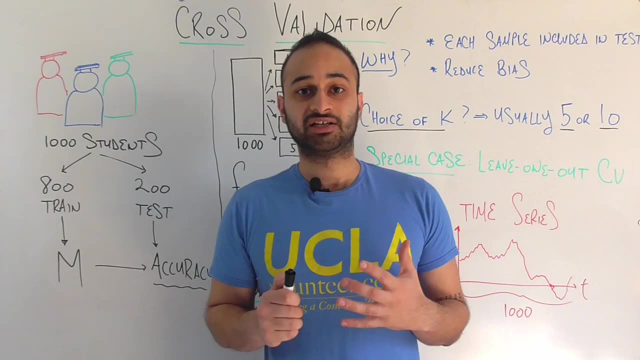 use 80% of the data for training and 20% of the data for testing. So what that means is 800 students randomly get assigned to training and the other 200 students will be used for testing the strength of the model that we build. So 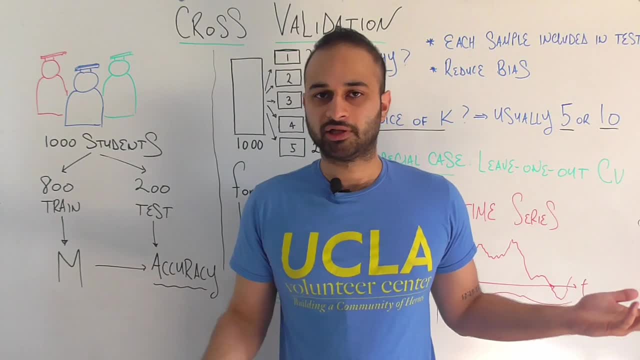 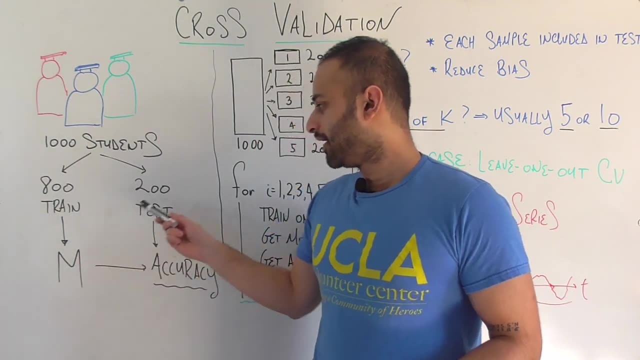 we go ahead and train our model On these 800 students. it doesn't matter what the model is For this video. it could be a random forest, a SVM, whatever, But we have a model M. Then we go ahead and apply this model M to these 200 test students which the model has not seen. 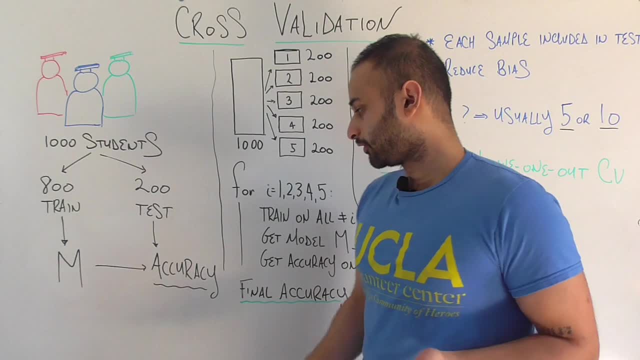 yet And we get a measure of the strength of the model. Let's just keep it simple and say: we calculate the accuracy And that should be the end of the story, right, It seems. we see if the accuracy is high or low, and then we go from there. 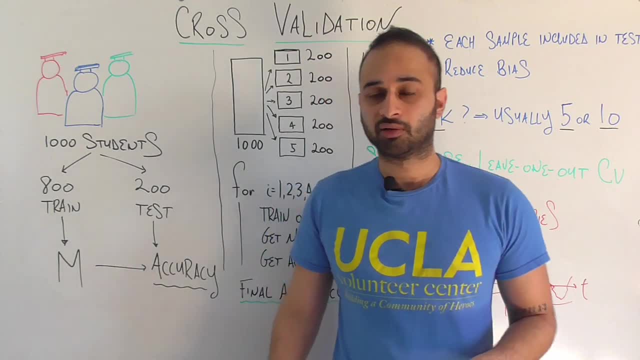 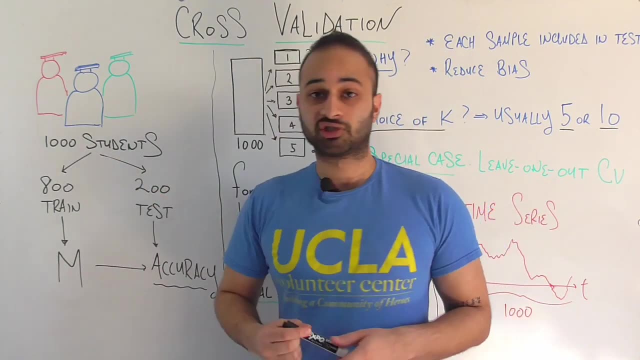 Well, this is okay. This is a good start for machine learning, But there are some key flaws with this idea. One of the key flaws with this idea is that it's not every student in the set of thousand students that we were using gets included in the testing set, So what that means is that we are only evaluating the 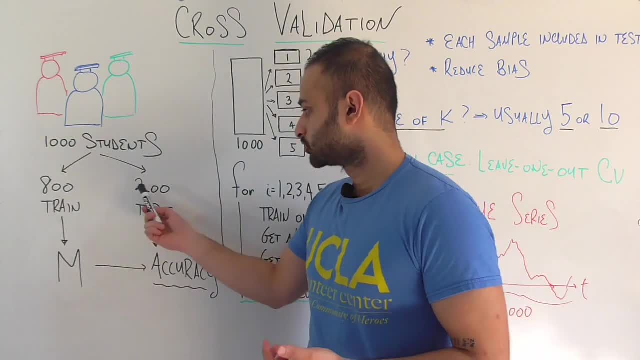 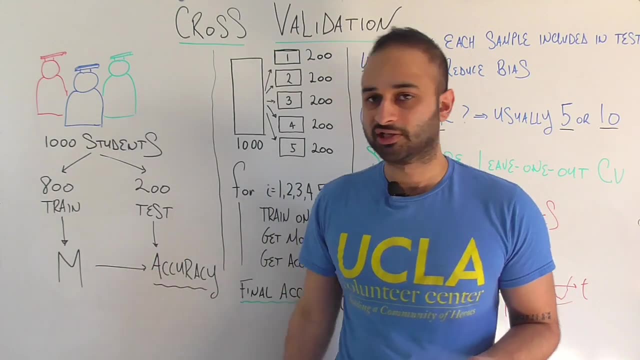 strength of our model on these 200 students. We haven't made any attempt to evaluate the strength of our model on the other 800 students And we can't using this model because that would contaminate the testing and training set. So we have to come up with a little bit of a more clever idea. The other big 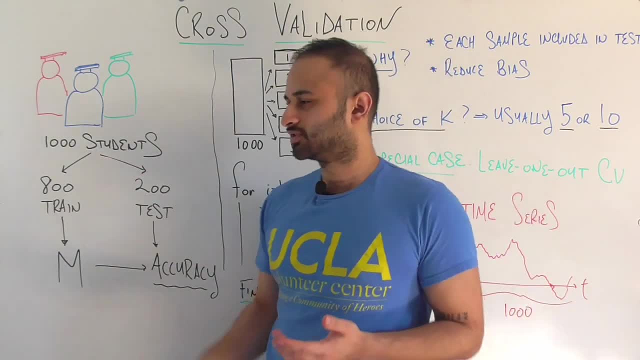 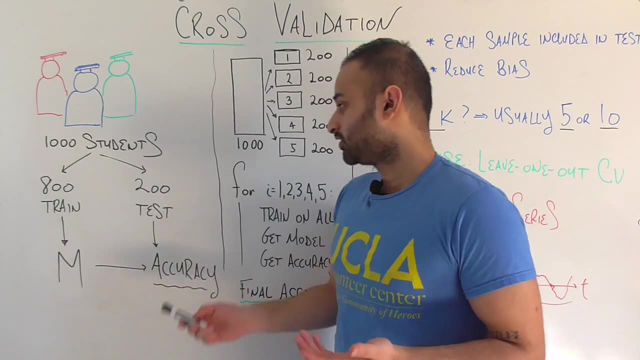 problem is that although our sample size is somewhat big, it's not that big And, especially for sample sizes even lower than our model, we don't want to have a than this. you might run into issues where, based on whatever randomness happens and whatever, 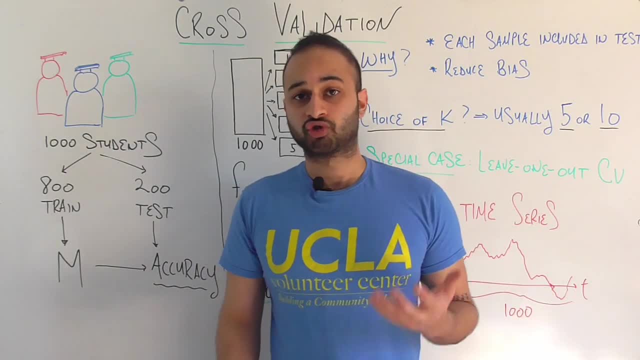 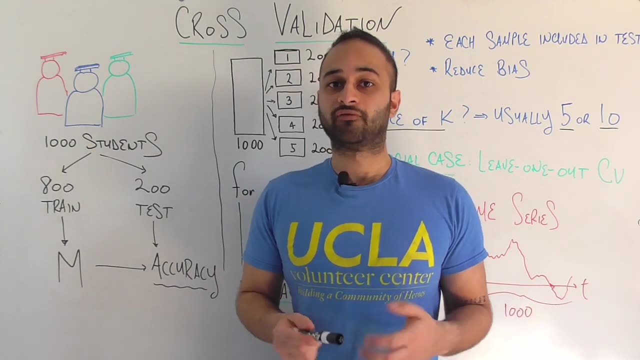 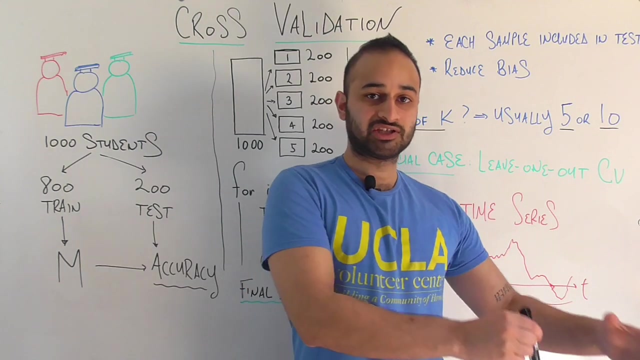 test set you get. the accuracy you're getting here might not be a true indication of the accuracy for the overall population. So we want something more robust, and that's where this idea of cross-validation comes in. So let me go ahead and just show you a concrete example of cross-validation, then I'll generalize. 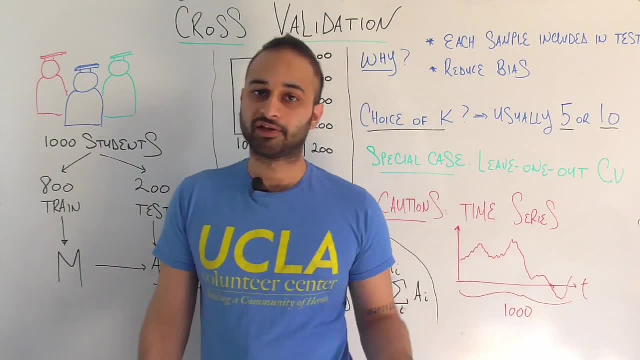 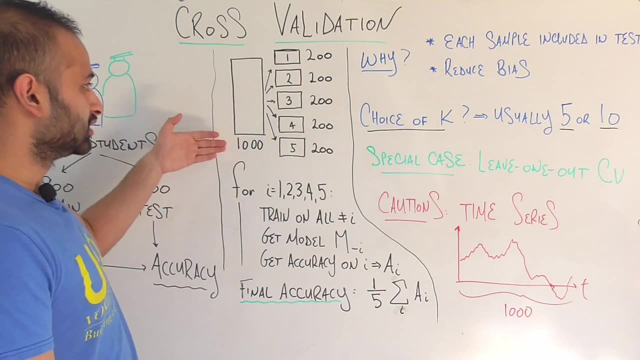 it a little bit and I'll show you some extensions and some cautions with cross-validation. So here's the new idea that we're going to use to make this example more robust. We're going to take our set of thousand students and we're going to split them into five groups. 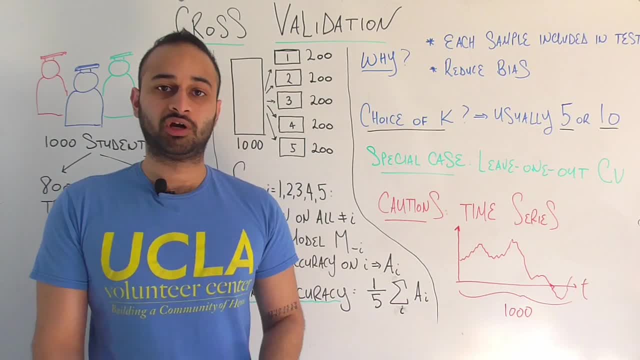 at random and each group is going to contain roughly the same amount of students. So here we're going to have 200 students per group. Now what we do is, for each i is equal to 1,, 2,, 3,, 4, and 5, we're going to train on all. 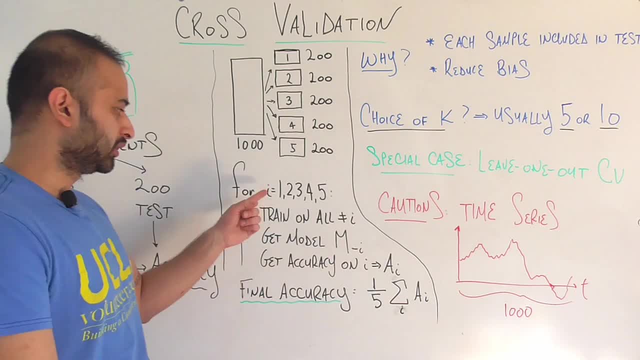 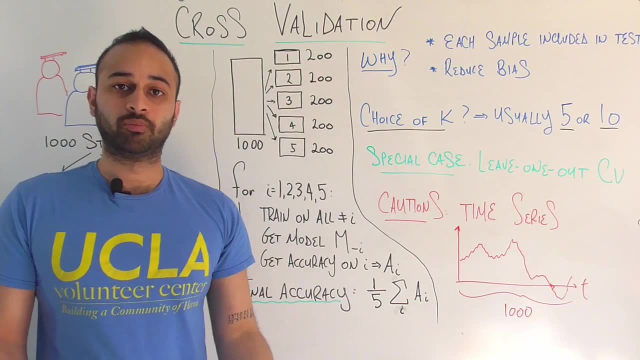 of the sets where it's not equal to i. So just to be concrete, the first thing we're going to do is say i is equal to 1.. So we're going to say group 1, this set of 200 randomly chosen students in group 1 will. 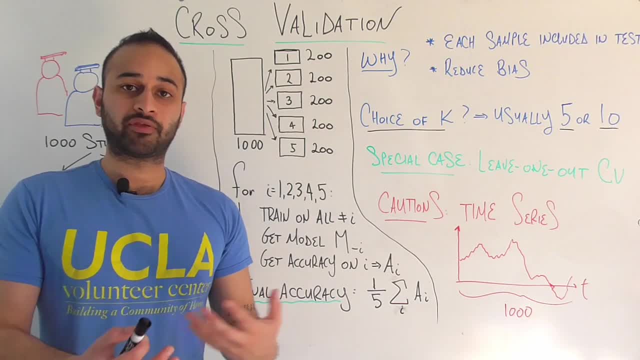 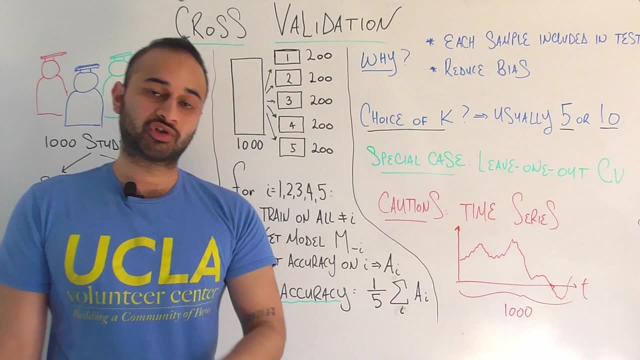 be our testing set And we're going to train the model on the other 800 students who are made up from group 2, 3, 4, and 5.. So far, this is the exact same thing we were doing back there. we're training on these. 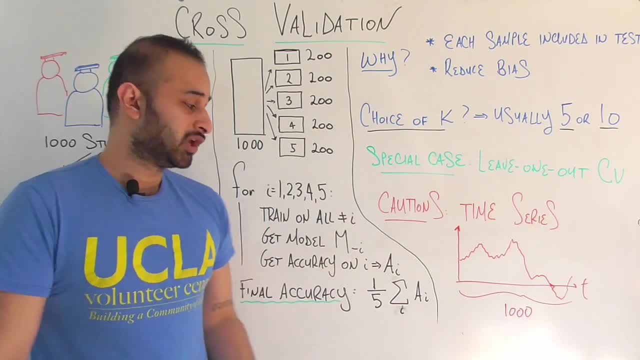 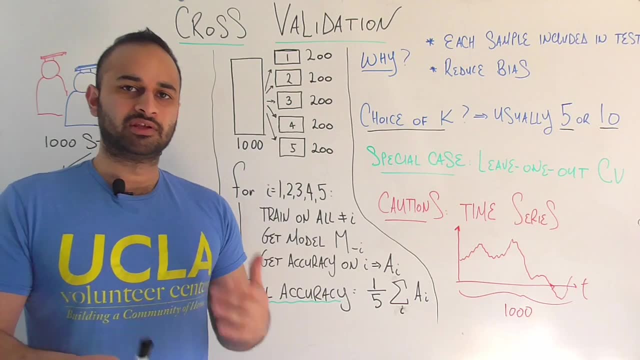 random 800 and we're testing on a random 200.. So then we build this model. we're going to call this model m sub-negative i. you'll see this notation sometimes. what it typically means is that this model is built on everything. 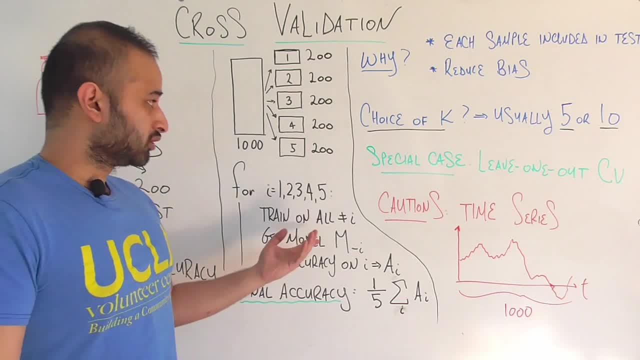 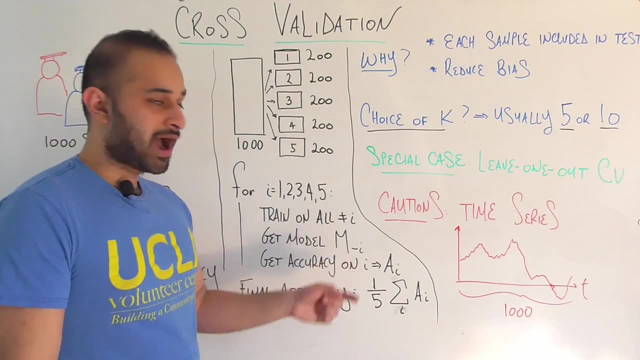 except set i, which is exactly what it is. We built this model using sets 2,, 3,, 4, and 5, so we'll call this model m-negative 1.. We get the accuracy on set i, which would be 1, here, and we would call that a sub-1.. 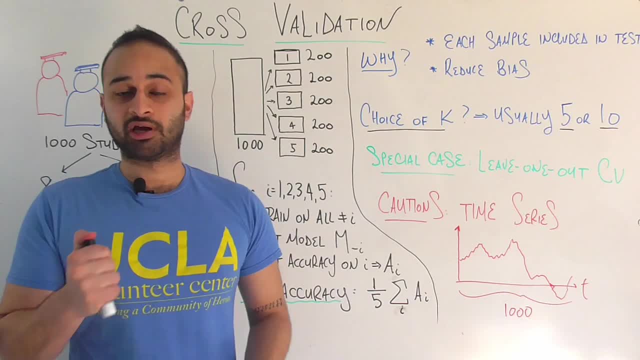 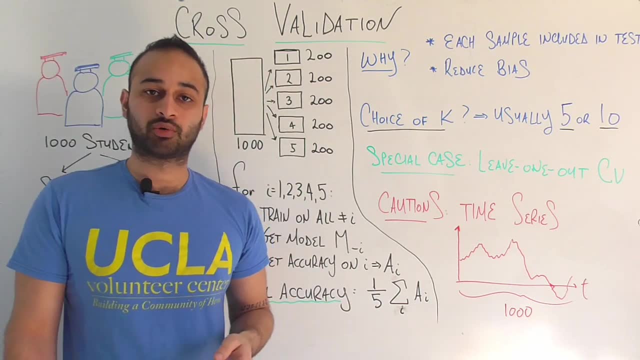 So so far, that would be the same exact procedure that we just did. now. here's where this becomes cross-validation and where it becomes more interesting. The next thing we do is say that now set 2 is going to be our testing set, so we're going. 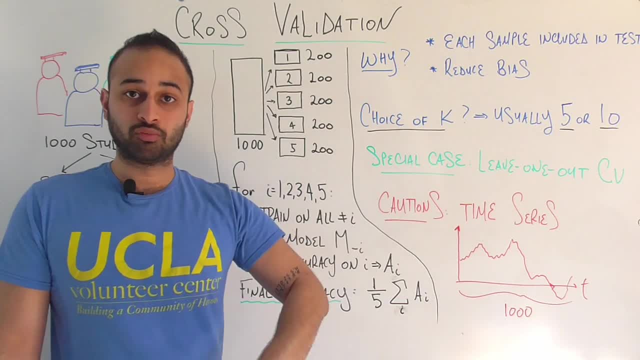 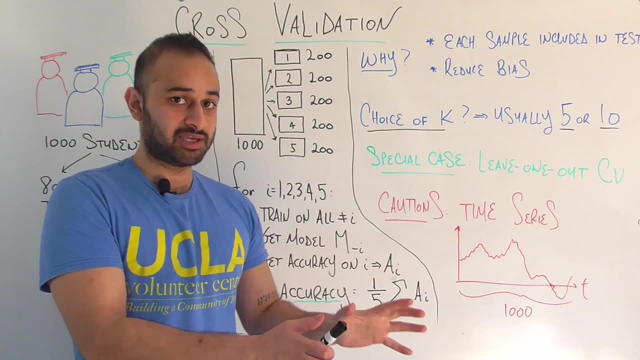 to pretend the model cannot see set 2,. we're going to train a new model on the 800 students that are made up from set 1,, 3,, 4, and 5.. So that's going to be a different model. just making that clear because we're using a different. 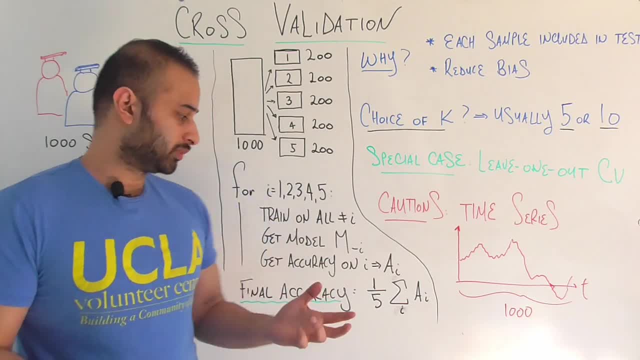 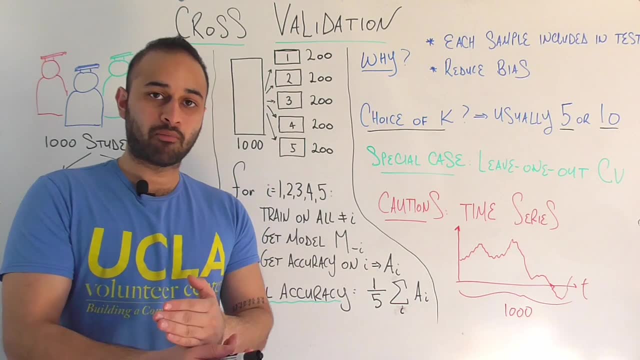 set of students to train this model, And then we're going to get that model, which will be called m-negative 2, since it has not been trained on set 2, and we're going to get the accuracy, using that model, on the students. 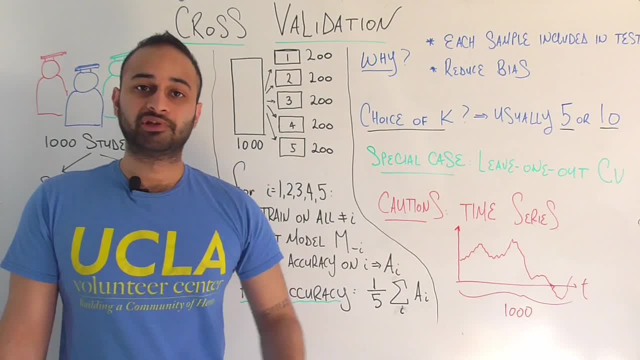 who are in set 2, and that's going to be called a sub-2.. And you can probably see where I'm going with this. the next thing we would do is call set 3, our testing set, and train the model on 1,, 2,, 4, and 5, and we go from there. 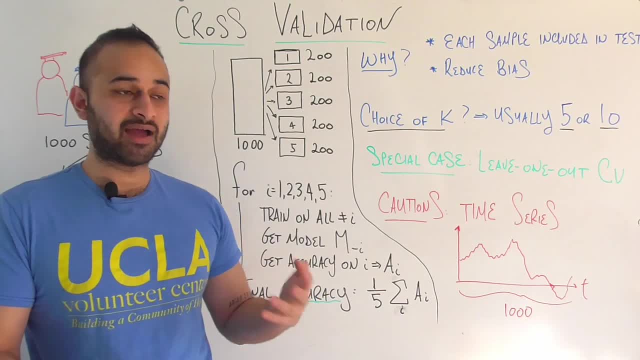 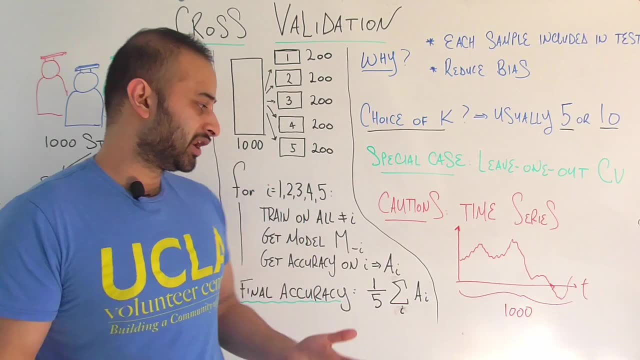 So, at the end of the day, we have 5 different models that were trained on 5 different subsets of these 5 sets that contain all of the students, And in order to get our final measure of accuracy here, we would go ahead and simply: 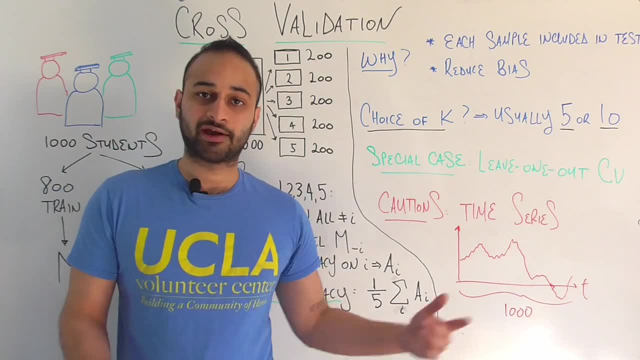 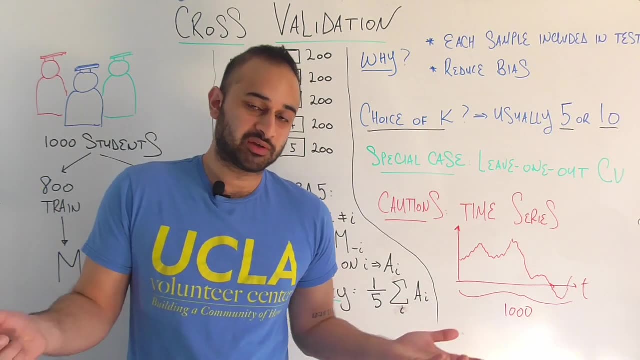 just take the average, so 1 fifth of the sum of all of these accuracies that we collected in this process. Now why is this a good idea? One thing I'll say off the bat is it's more computationally expensive, right. 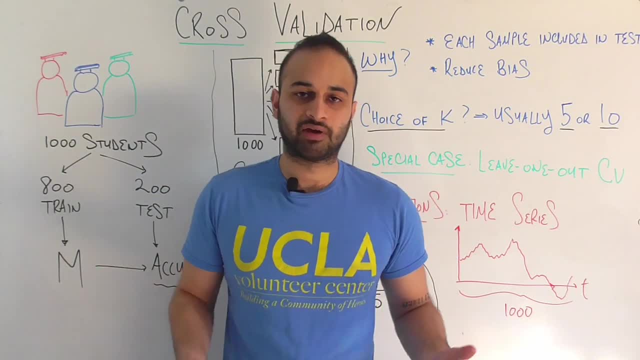 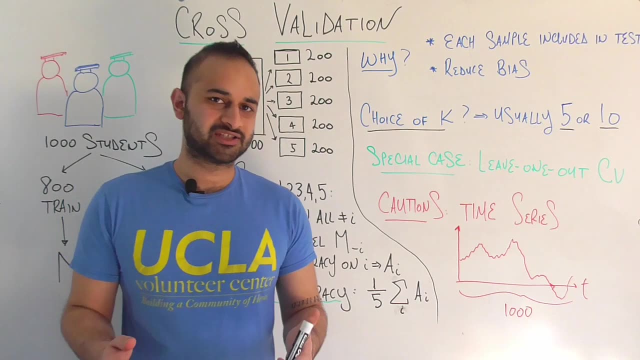 If your model here took like 5 hours to train, just for example, if you have lots of students or something, this is going to take 5 times longer than that because you're building 5 models here. Of course it's computationally more expensive, but why is this still a really good idea and 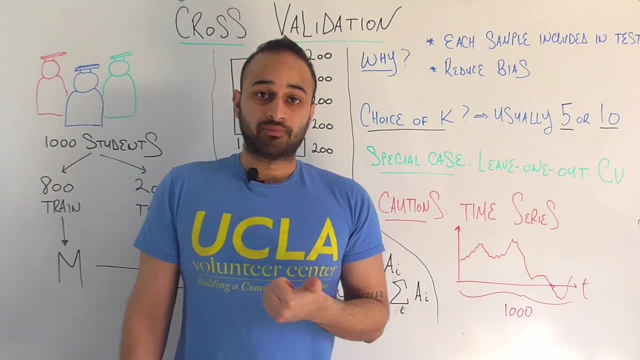 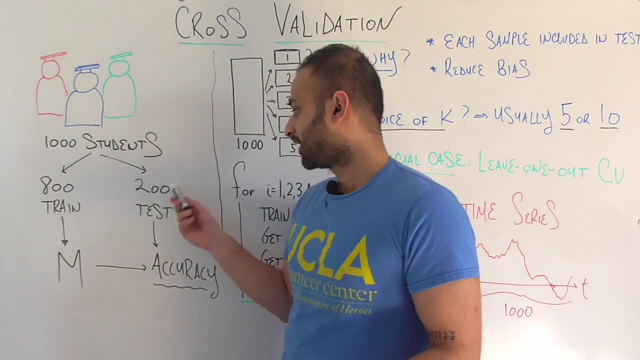 why is this something that people do really often in practice? So one of the big problems that we addressed- that we didn't address here- is that every student gets included in testing at some point. So, whereas before we only had this set of 200 students getting tested on in order to 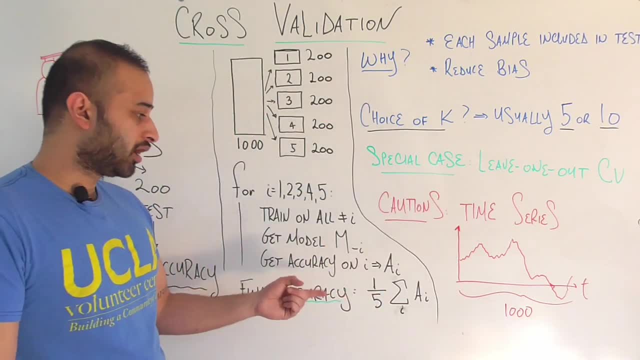 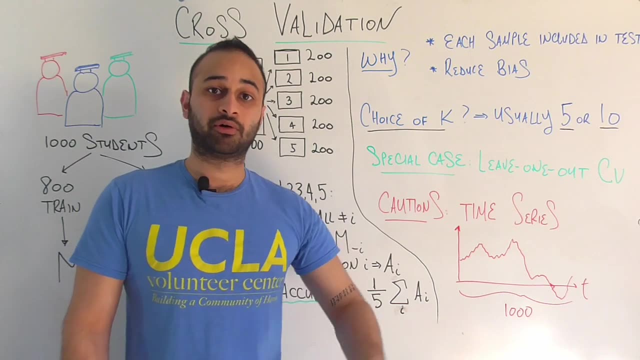 determine our accuracy now in our calculation of final accuracy, we are testing every single one of these thousand students because, remember, each of these sets gets used as the testing set at some point or the other, which means that every student in each of those sets gets. 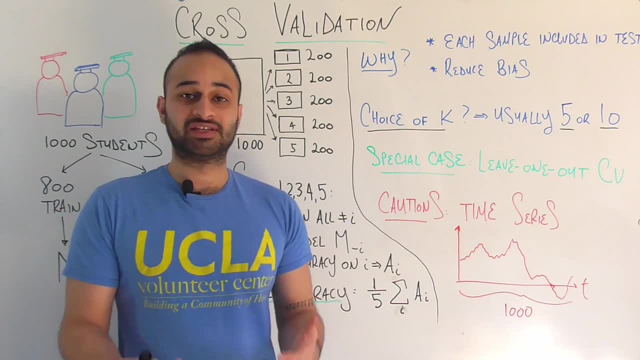 used as a testing example, Which means that our final accuracy is truly combining all of these sets, And that's what we're going to do here. So we're going to go ahead and take a look at our final accuracy and we're going to 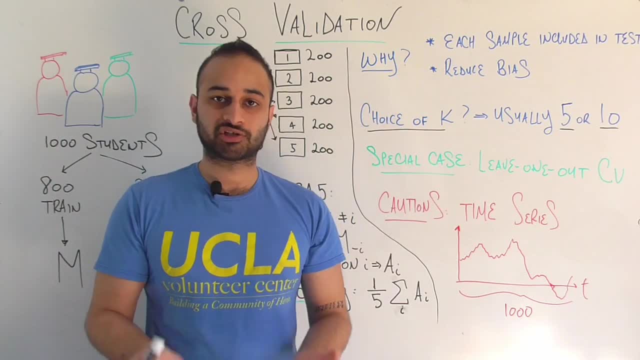 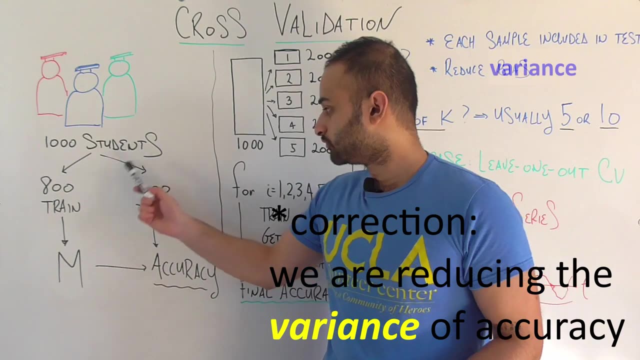 see that we're reducing the strength of our models on all of the students in the dataset. So that's one big pro. An even bigger pro is that we're reducing the bias. So something I said earlier was that this set of 200 students, although it is random, 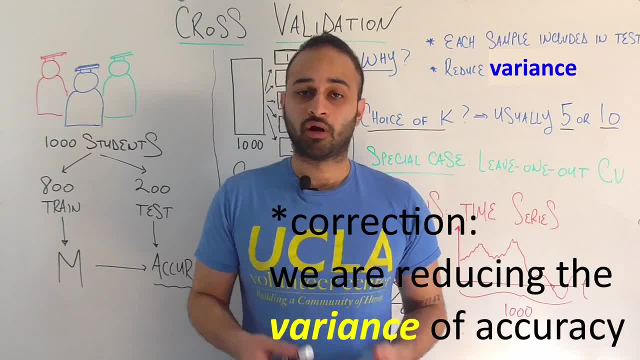 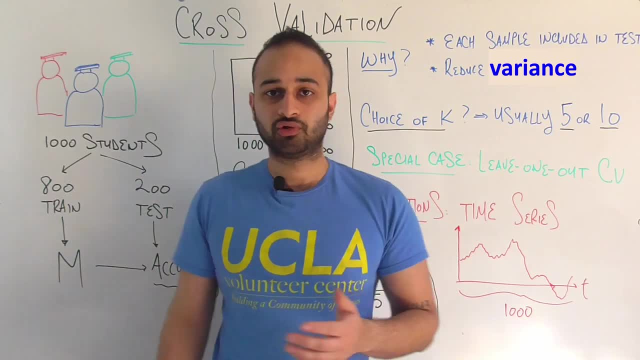 it could be better or worse than the true performance of the model on the general population. Here we are reducing that bias. I'm saying alright, I'm not going to go ahead and use the model on just one set of 200 students. 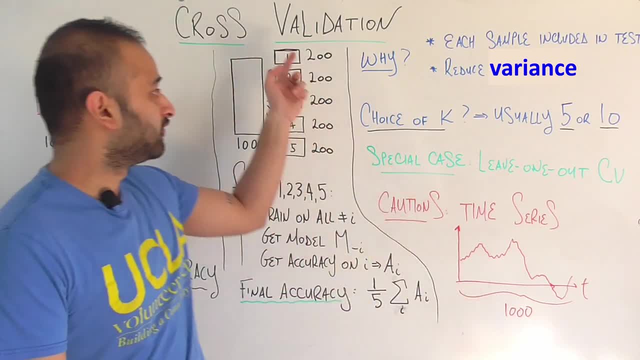 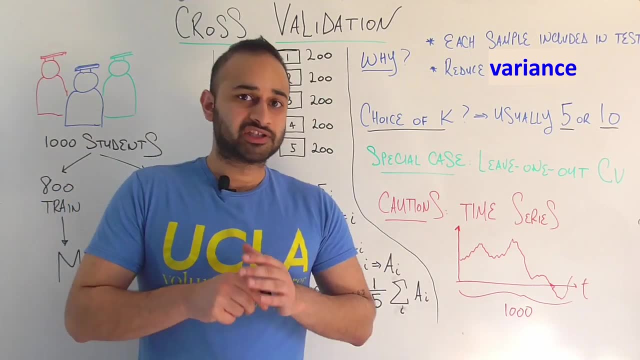 I'm going to build 5 separate models and test them on these 5 different sets of 200 students, So we start getting a better idea of the true strength of this model that we are building. Of course, now let's say a new student comes in, a completely new student that you've never. 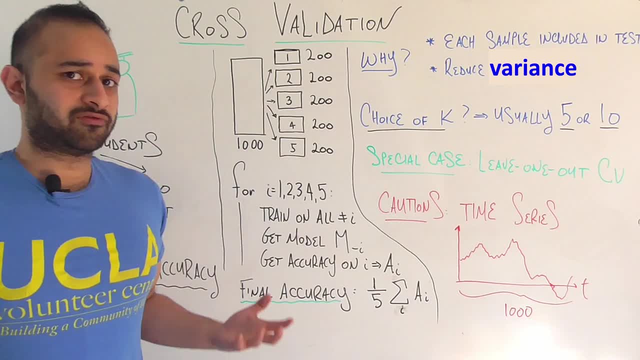 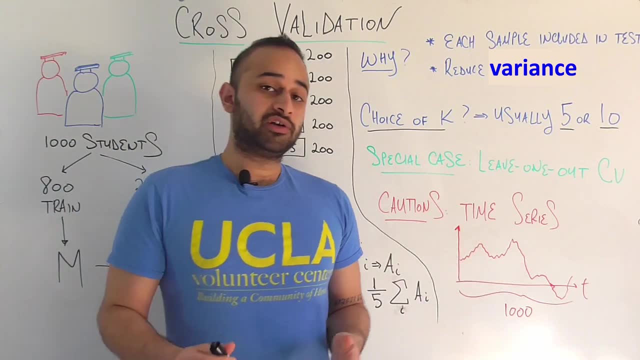 seen before. Which model do you use? Because, if you've noticed, we've built 5 models here. One for each combination of training sets right. So which model do we use to predict this next student? Well, here, you typically combine the models in some way. 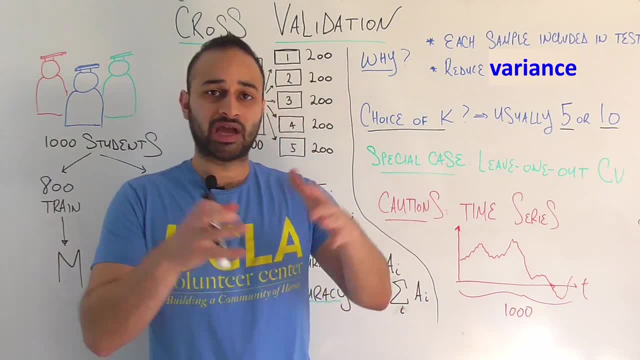 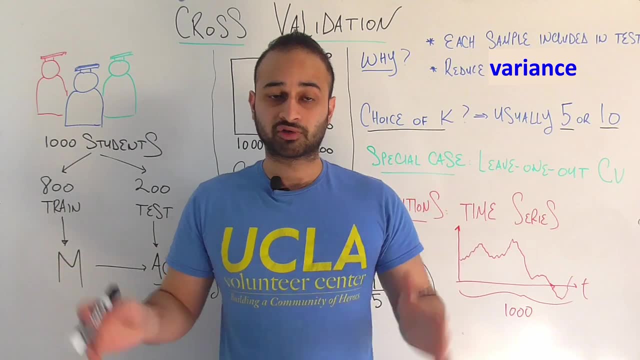 Here it's a binary classification problem, so it's relatively simple. Let's say that we have our 5 models: M-1,, M-2,, M-3,, M-4, and M-5.. And let's say that 4 of these models predict that this new student will drop out of their 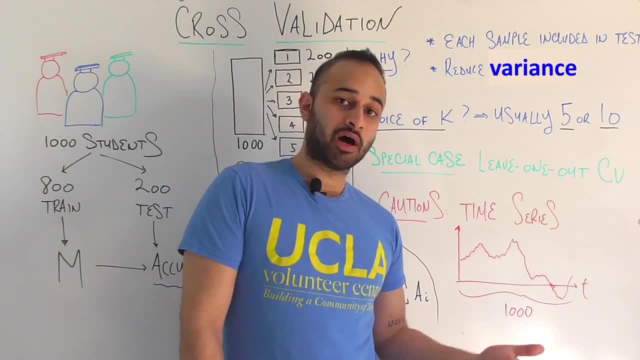 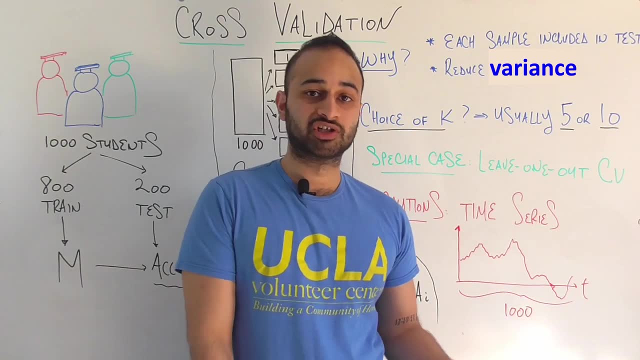 major in the next semester and the last model says that they will not. We can just do a simple majority and we can say that the prediction for this student is that they will drop out. If you're doing a regression example, you could just take a literal arithmetic average. 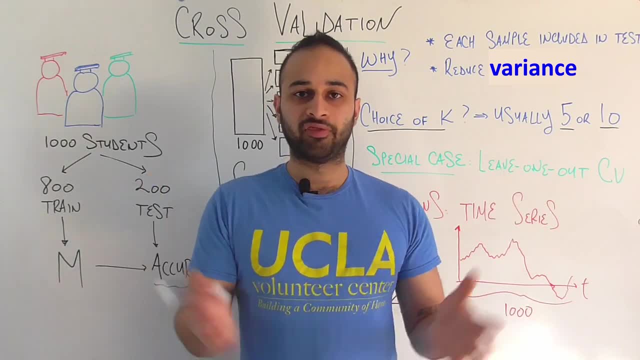 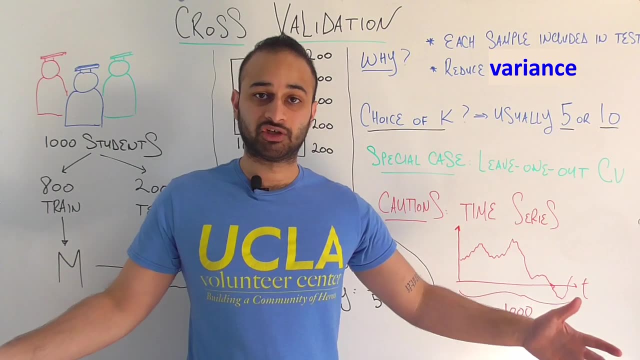 of your predictions from the 5 models and so on. So you're going to combine the models in some way to get your final model. Now I'm ready to finally put a name on this procedure. This is called k-fold cross-validation, And here our k was equal to 5.. 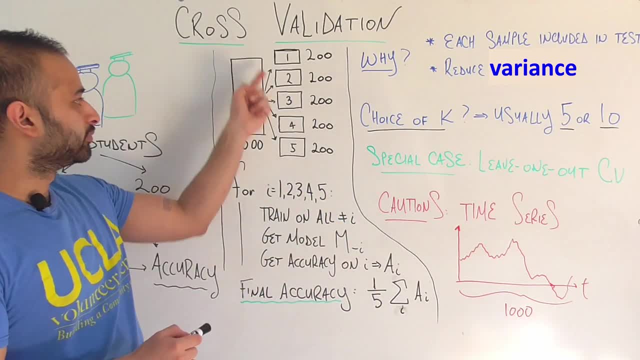 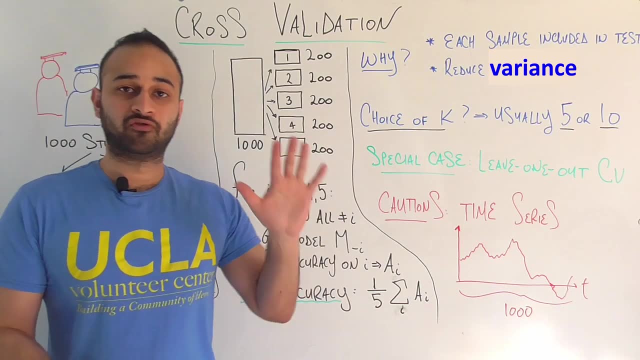 And k is the number of sets that you break up your whole set into. So it's called 5-fold cross-validation for us, because we took our initial set of 1000 students, broke it into 5 sets and then went from there. 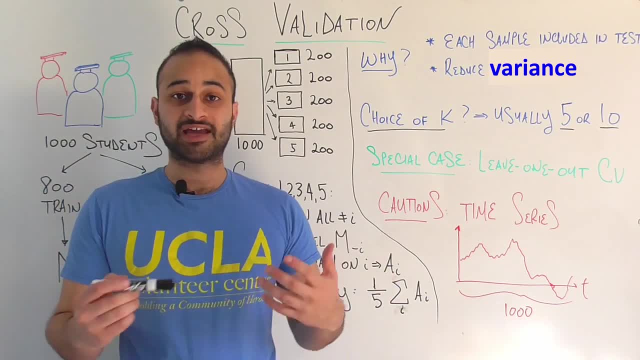 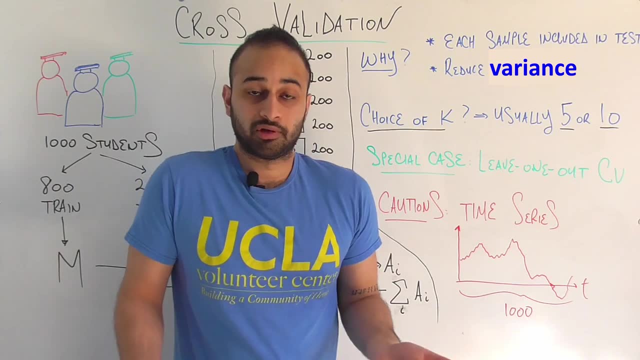 If we had broken that into 10 sets of 100 students each, this would be called 10-fold cross-validation, And actually 5 and 10 are the typical numbers that people use in practice, but there's no rule. You can really use whatever you want that you think is appropriate for your application. 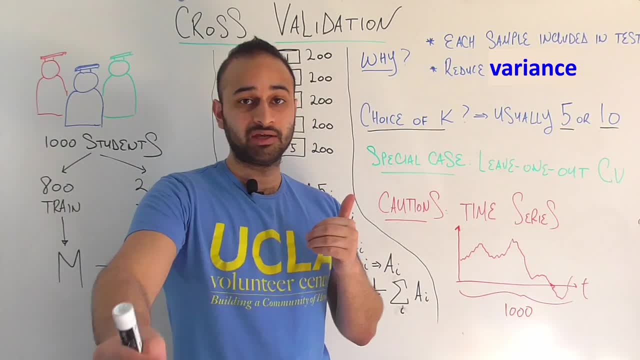 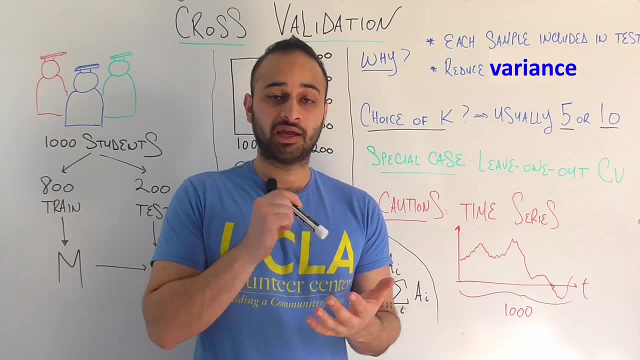 But it is important to think about the trade-offs. If you make k way too big, that means that you're going to split up your initial set into many, many, many, many sets. That means every time you are testing a model, you're only testing it on a little bit of. 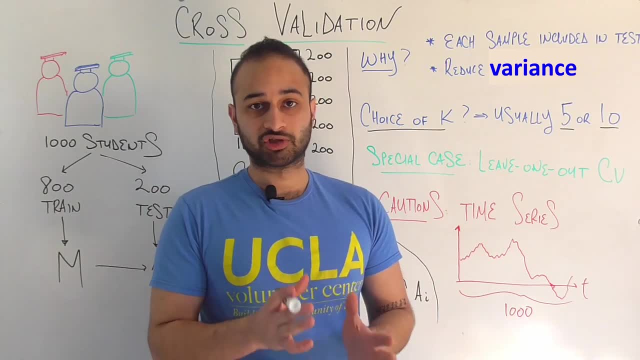 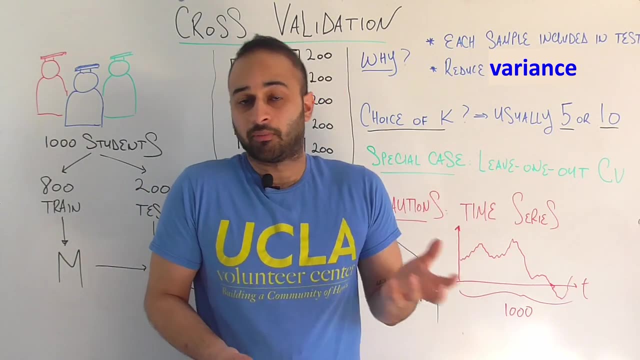 samples. However, if you make your k too small- like, let's say, use k is equal to 2, then essentially you're just taking your entire sample of students, splitting it in half and you're only training on half. So that might or might not be appropriate. 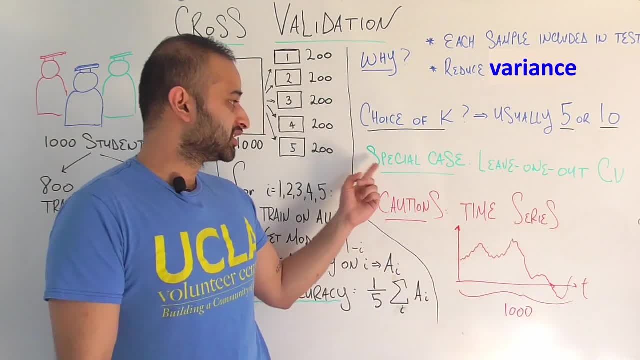 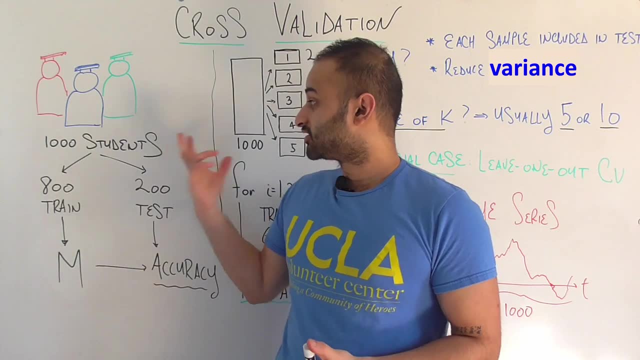 So just think about your choice of k Again. typically it's 5 or 10.. A very special case of cross-validation is called leave-one-out cross-validation, And this is a very interesting case. It basically says that I'm going to take my sample of a thousand students and I'm going 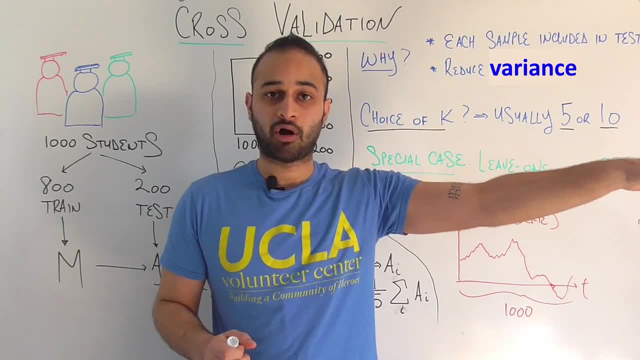 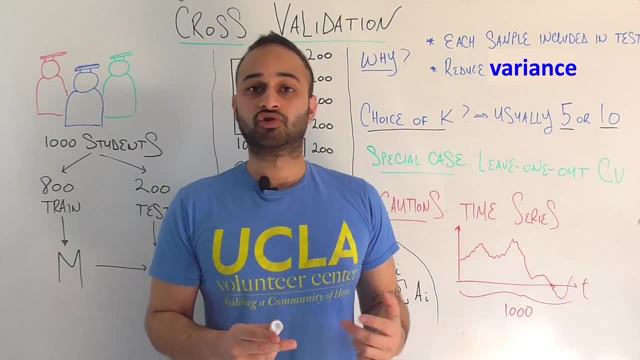 to take one student and leave them out each time, and I'm going to train my model on the other 999 students and then take that model and apply it to the one student that I had left out. Then I'm going to train my model on a different set of 999 students and test it on the one. 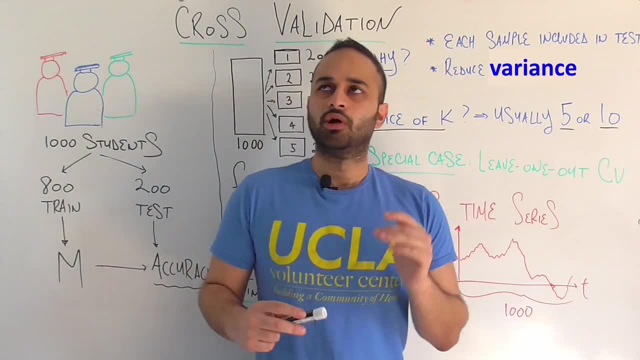 student I left out, And you basically do that a thousand times. So one thing to note is that this is going to be very computationally expensive because you have to train not five but a thousand students, So that's a very interesting case. 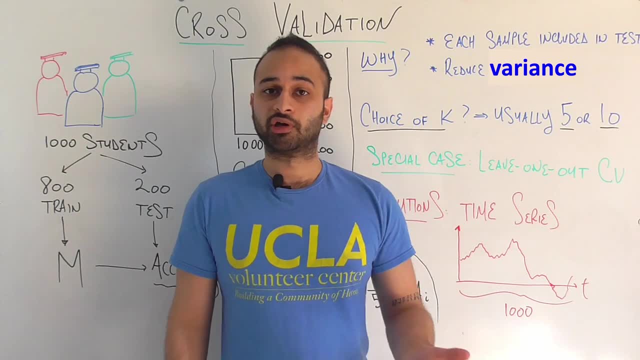 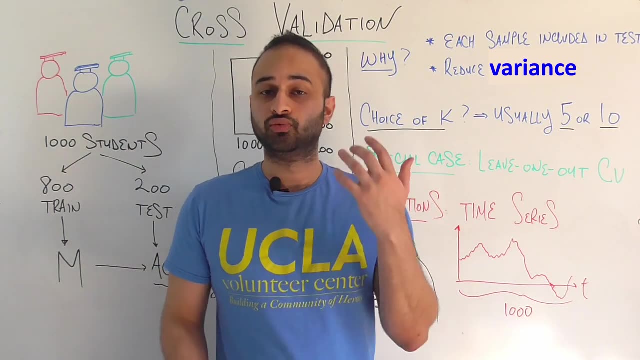 But this is also an option that is available when you're doing cross-validation. And the very last thing I'll say: because we talk about time series so much on this channel, and just because I'm a big fan of time series, you have to be careful when you're.